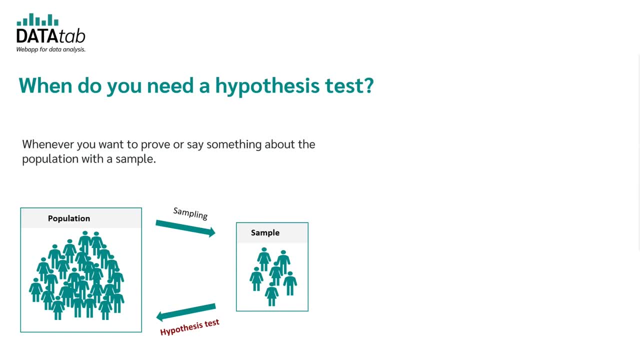 value or the standard deviation of different variables in order to describe your sample. But in our example now we want to make a statement about the whole population, so we use our sample and with the help of a hypothesis test, we can infer the population. So the goal of a hypothesis- 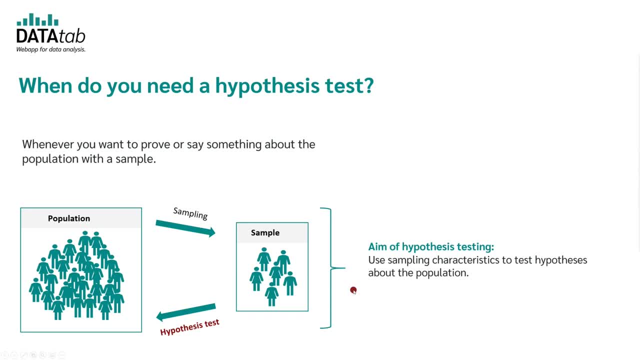 test is to test hypotheses about the population based on sample characteristics. So you have a sample and with the help of this sample and with the appropriate hypothesis test, you can determine whether there is a difference in the salary of men and women. But before you can calculate a hypothesis test, you have to make sure that your hypothesis is 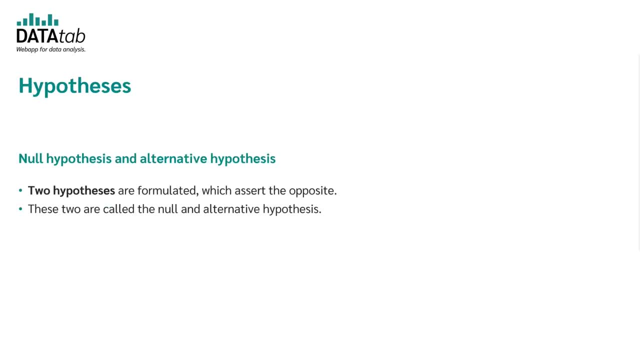 formulated correctly, and we're going to talk about that now. When you want to formulate a hypothesis, there are always two hypotheses that assert the opposite. These two hypotheses are called null and the alternative hypothesis. Therefore, the null and the alternative hypotheses always claim exactly the opposite. Usually, the null hypothesis assumes that there is no difference between two. 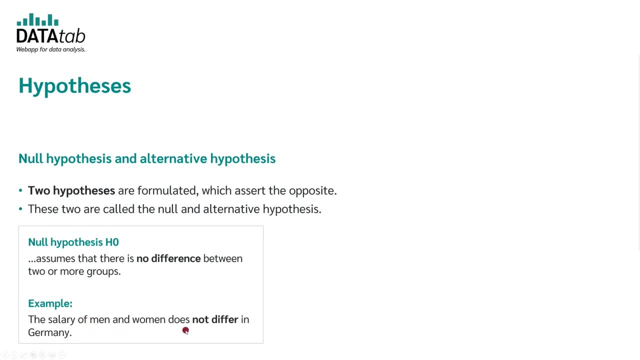 groups. So, for example, the salary of men and women does not differ in Germany, and the alternative hypothesis assumes that there is a difference. So, for example, the salary of men and women differs in Germany. Furthermore, there are certain types of hypotheses and in order to formulate your, 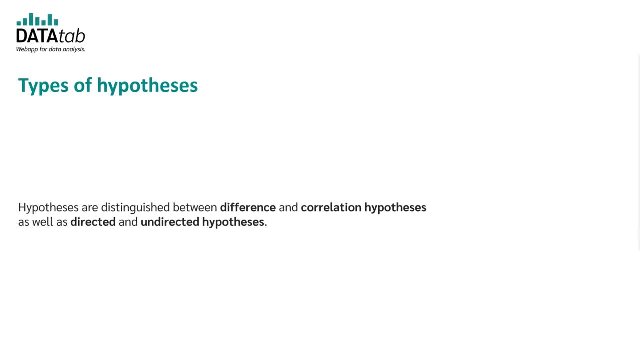 hypothesis and in order to find the right test, it is very important that you know these types. Generally, we can distinguish between difference and correlation hypothesis, as well as between directed and undirected hypothesis. So, for example, the difference and the correlation hypothesis. areقةßar, The rate of success or loss in Germany is significantly different from that fellowsной. 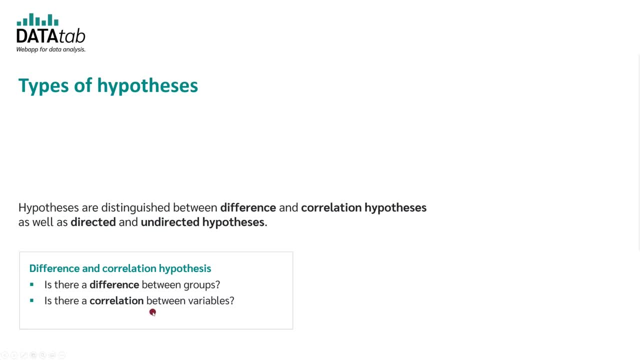 a difference between groups or is there a correlation between variables? And when we look at the directed and the undirected hypotheses, we can ask the question: is there a difference or a correlation? And is there a difference or a correlation in a certain direction when we have a directed? 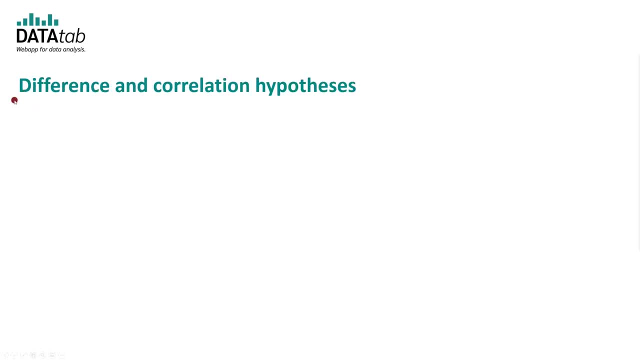 hypothesis. So let's take a closer look now at the difference and the correlation hypotheses. We start with the difference hypothesis. A difference hypothesis checks if there is a difference between two or more groups. So in our example we have the group of men and the group of women and we want to investigate. 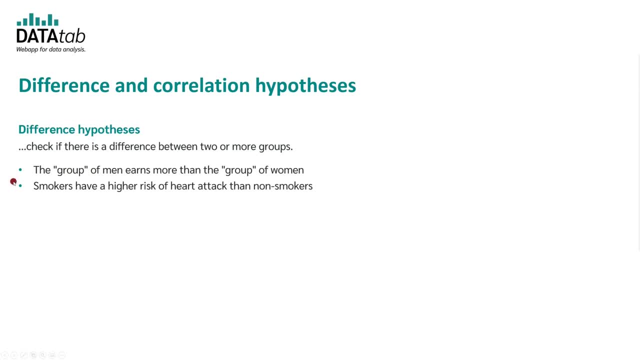 if the group of men earns more than the group of women Or, for example, smokers have a higher risk of a heart attack than non-smokers. So we always want to look at the difference between two groups In order to formulate a difference hypothesis. we need a categorical variable, for example: 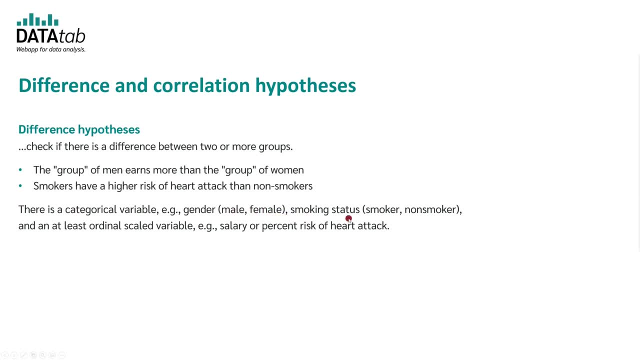 gender, where we have male and female, or also the smoking status, where we have smokers and non-smokers, and at least one ordinal scaled variable, for example the salary or the percentage risk of a heart attack. Now let's take a look at the correlation hypothesis. 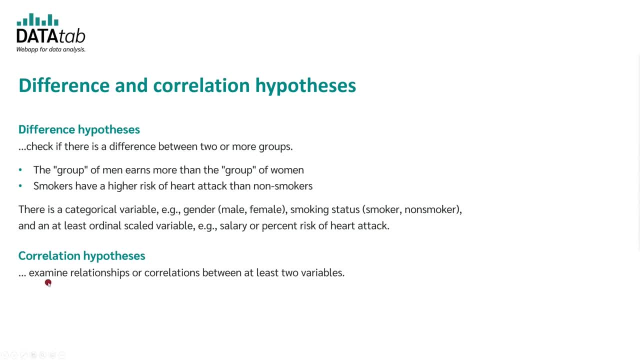 A correlation hypothesis wants to examine the relationship or the correlation between at least two variables. So, for example, the bigger a person is, the higher he or she is, which would be the correlation between the body height and the weight of a person. Or the more horsepower a car has, the higher the consumption of the car is. 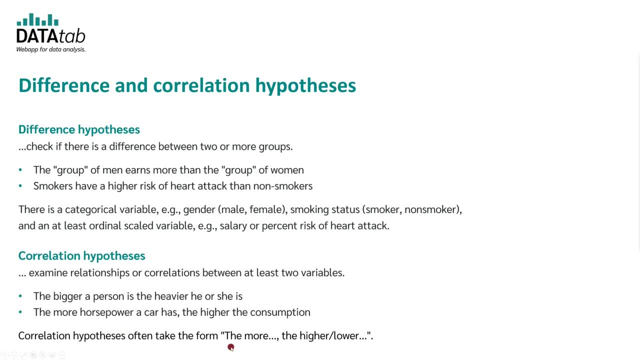 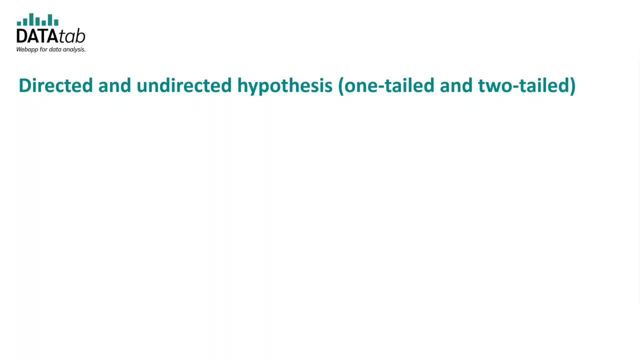 When you want to formulate a correlation hypothesis, You often take the form the more, the higher or the lower in order to formulate it. Okay, now let's take a look at the directed and the undirected hypothesis. What is an undirected hypothesis? 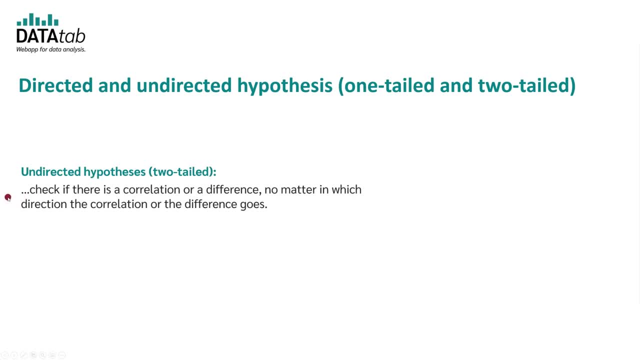 An undirected hypothesis wants to check if there is a correlation or a difference, no matter in which direction the correlation or the difference goes. So, for example, There is a difference between two groups. There is a difference between the salary of men and women. 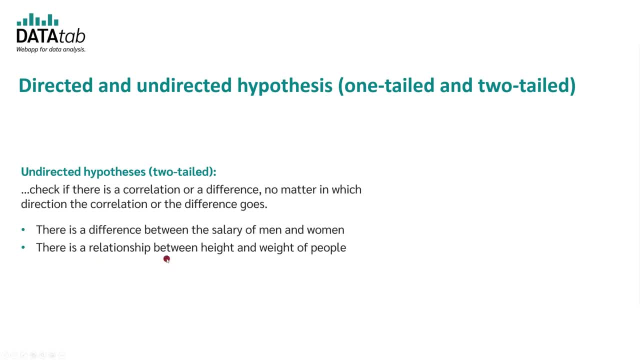 Or another example: there is a relationship between height and weight of people. If we now look at the directed hypothesis, we can see that the directed hypothesis additionally indicates the direction of the correlation or the difference. So, for example, men get the higher salary than women. 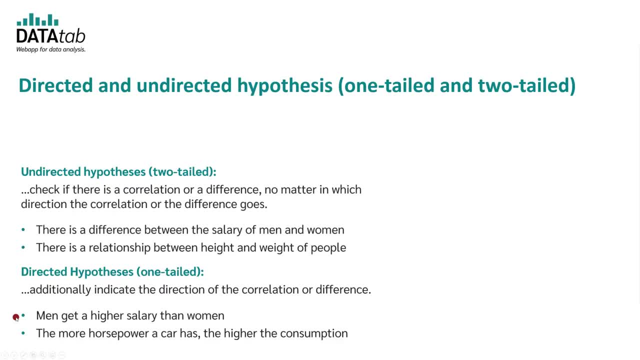 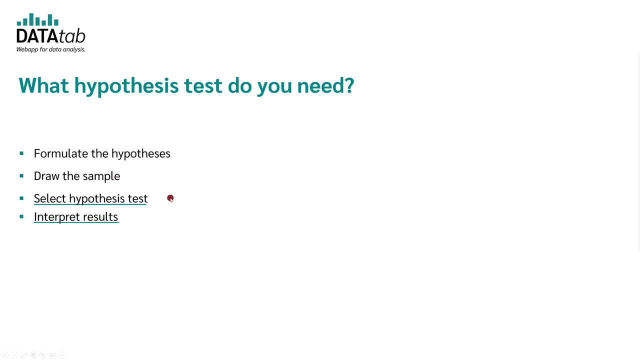 Let us now come to the question: which hypothesis test we need. We started with formulating the hypothesis, We talked about drawing the sample, And now the question is: which hypothesis test should we select? In order to find it out, you can use DataDap. 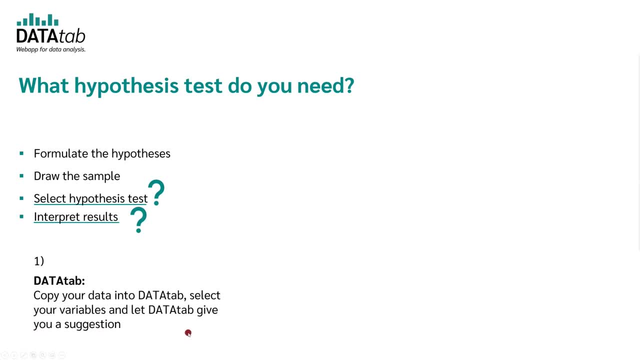 You can copy your data into DataDap, select your variables and then let DataDap give you a suggestion for the right hypothesis test. If you want to get more information About correlation, You can also look at the video descriptions. When talking about hypothesis tests, it is very important to also look at the probability. 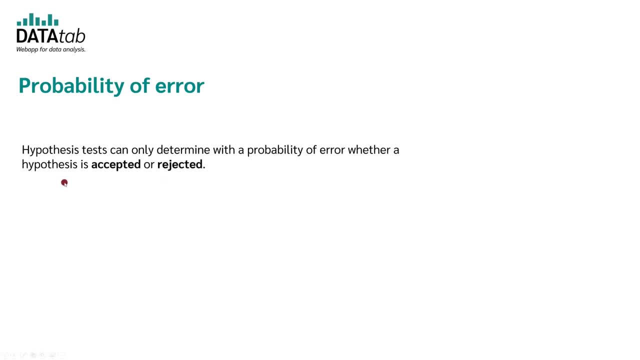 of error. The probability of error is important because hypothesis tests can only determine with a probability of error whether a hypothesis is accepted or rejected. So let's look at an example. We have two samples here, Sample 1 and sample 2.. And they differ from each other. 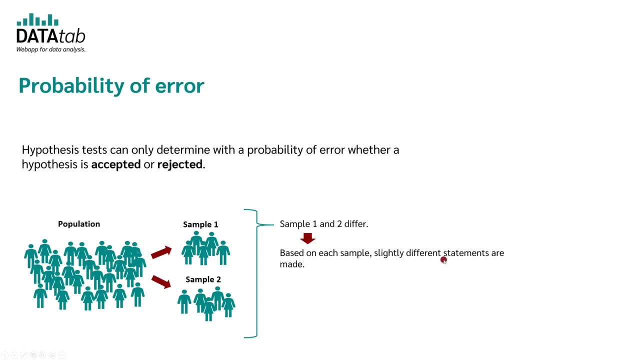 So, based on each sample, we get slightly different statements about the population. In the worst case, we would draw a sample that is very different from the population, And this may cause us to make an incorrect statement about the population. Let's now look at the p-value. 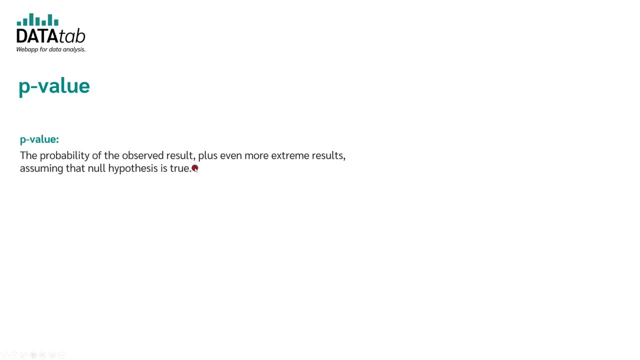 What is the p-value? The p-value is the probability of the observed result Plus the probability of the observed result Plus even more extreme results, assuming that the null hypothesis is true. So this means that in the population we have women and men and we have no salary difference. 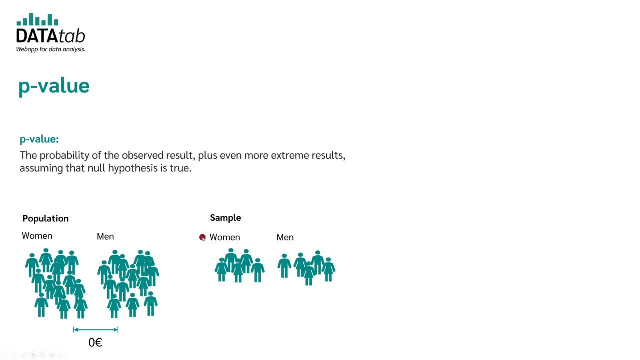 In our sample, we would, let's say, have a salary difference between men and women of 250 euros. So our assumption is: in a population, there is no difference in salary between men and women. And what does the p-value mean? The p-value tells us now. it tells us how likely it is to draw a sample in which the 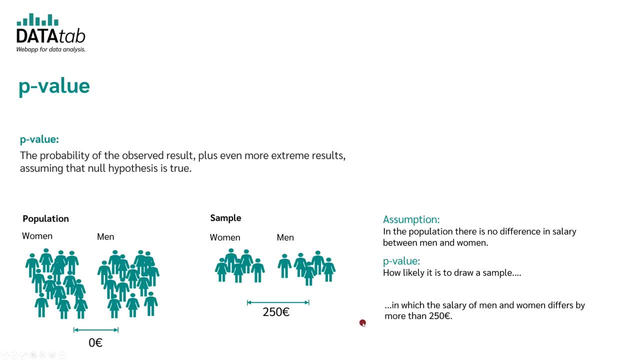 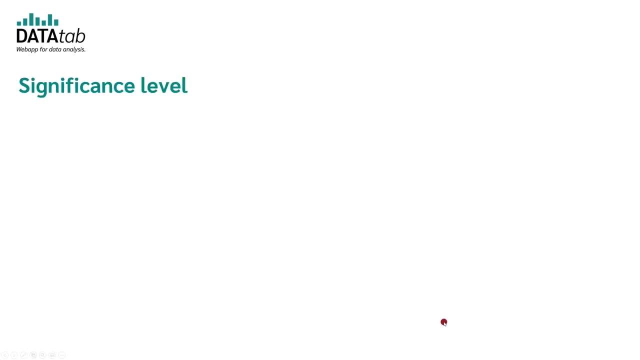 salary of men and women differs by more than 250 euros. Another very important aspect when we are talking about hypothesis tests is the significance level. The significance level is always determined before the examination and it may not be changed in order to obtain a desired statement. 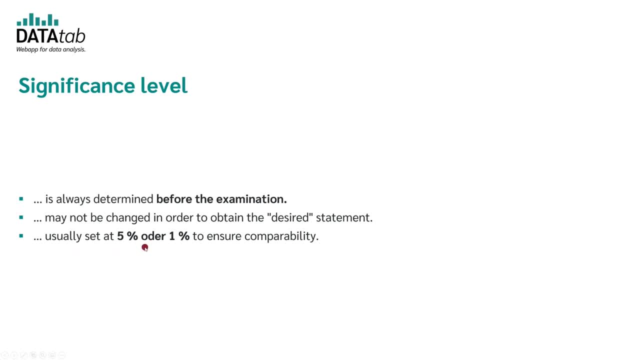 Usually The significance level is set at 5% or at 1% in order to ensure comparability. So if we have a significance level, also called alpha level, of smaller or equal 1%, we call it a highly significant result. If we have an alpha level of smaller or equal 5%, we say that result is significant. 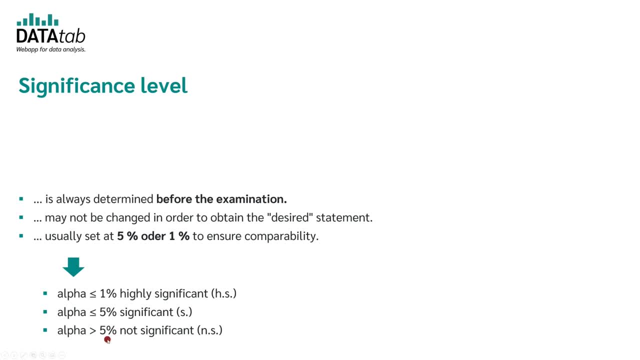 And if our alpha level or significance level of equal 1%, we say that our result is more significant. And if our alpha level is less than or equal to 1%, is higher than 5%, the result is not significant. So let's take a look at the. 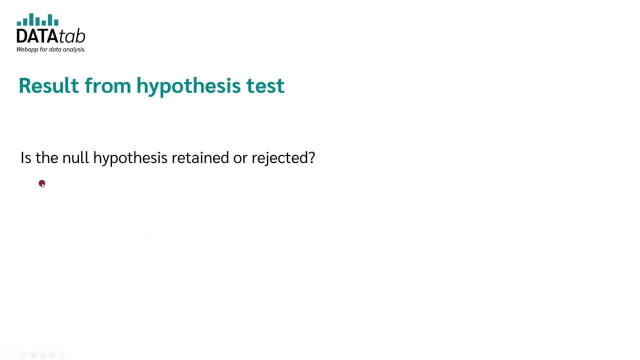 result of an hypothesis test now. So the question is: what should we do with the null hypothesis? Should we retain it or reject it? So first we set the significance level, then we calculate the p-value and then we ask the question: is the p-value greater than the specified significance level? If it is greater than, 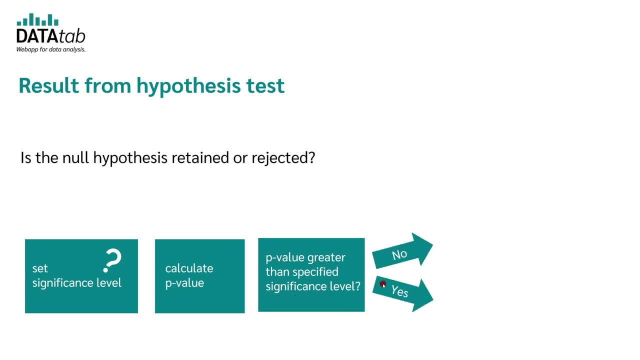 our significance level, we keep our null hypothesis. So, for example, we say, ok, there is no difference. If it is not greater than the significance level, we reject the null hypothesis. Ok, so whenever we are using hypotheses tests, we have a certain risk of errors. so we have certain 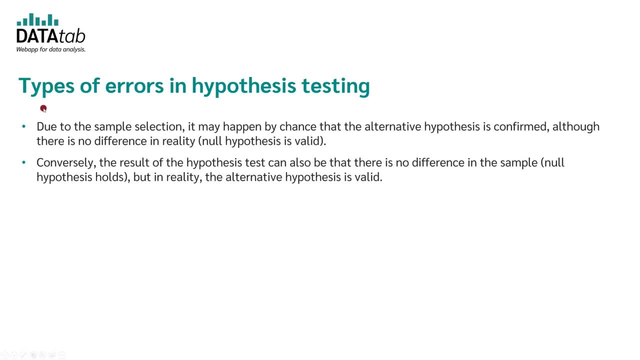 types. that is a greater trend than that of the кто is greater than or than the of errors in hypothesis testing Due to the sample selection. it may happen by chance that the alternative hypothesis is confirmed, although there is no difference in reality. So the null. 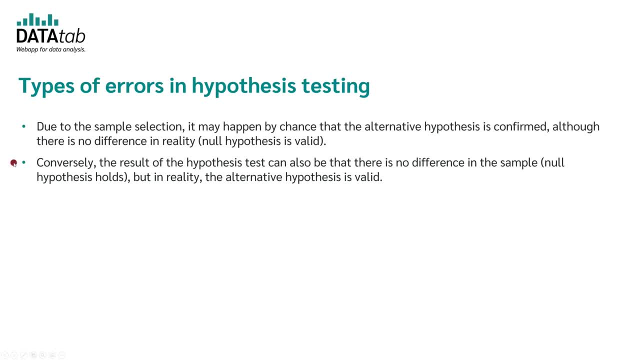 hypothesis is valid. Conversely, the result of the hypothesis test can also be that there is no difference in the sample. null hypothesis holds, but in reality the alternative hypothesis is valid. So we have the alpha error, type 1 error, which says that if the alternative hypothesis 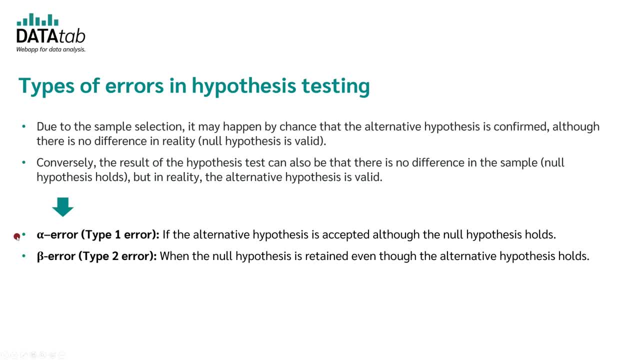 is accepted although the null hypothesis holds, and we have the beta error, the type 2 error, and we make the type 2 error when the null hypothesis is retained, even though the alternative hypothesis holds. So in this table you can see a summary of these. 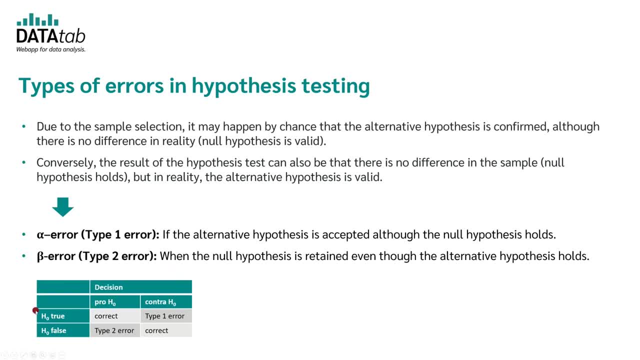 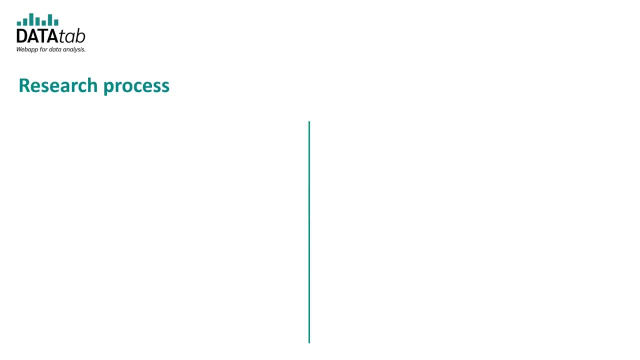 two types of errors and the decision we make. Okay, let's take a final look at the research process now. Well, in order to calculate a hypothesis test, we first have to define a research topic. Based on our topic, we write down our research question And from the research 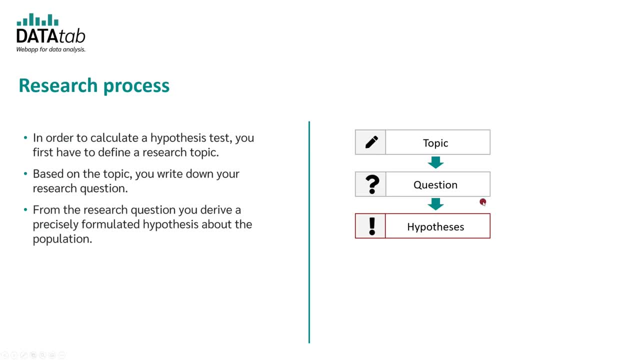 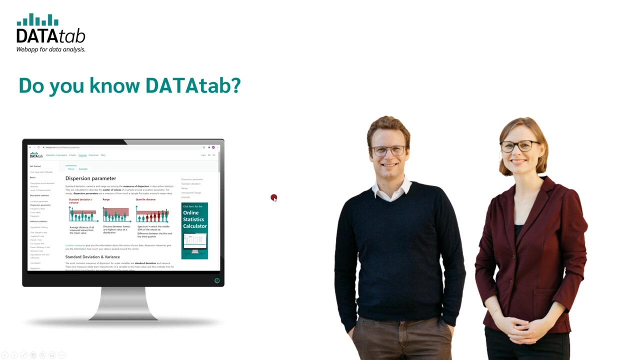 question, we derive a precisely formulated hypothesis about the population And, finally, we can choose a suitable hypothesis test based on the hypothesis in order to test our assertion. If you don't know Datadep yet, just have a look at datadepnet. And thanks for watching this video.